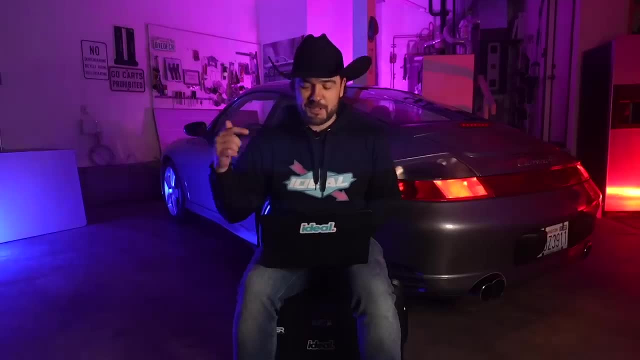 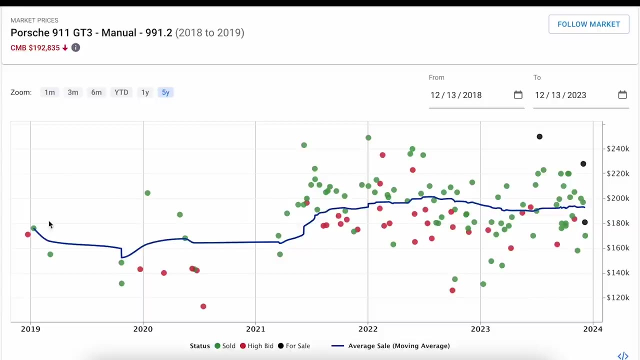 if you had bought one pre-pandemic. Now, guys, let's jump on the trusty dusty computer and take a look at a couple of the different markets and what was so crazy about them Here. first pre-pandemic: check out this like-new 1,100-mile one-year-old 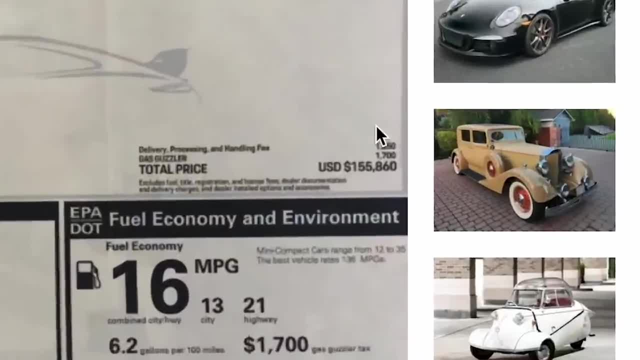 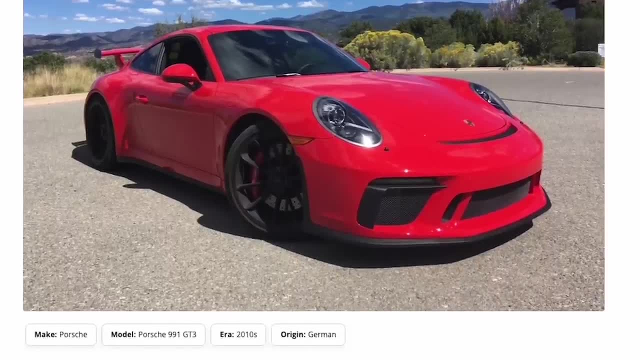 GT3 that sold for $130,000.. Now, if we take a look, MSRP was $155,000.. And given the discounts that I told you about the dealers giving pre-pandemic, the first owner probably paid $30,000. 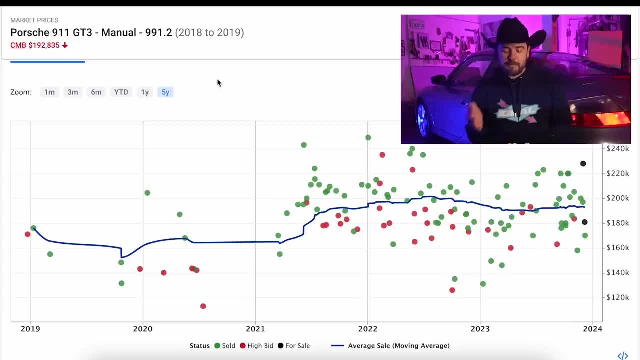 less and either broke even or even made a little bit of money on this deal. Now, if we go back to the chart, if you follow this average sales line, you can see only a few cars sold between 2020 and 2021.. And then, bam, in 2021, look at this cluster of cars all selling for $200,000. 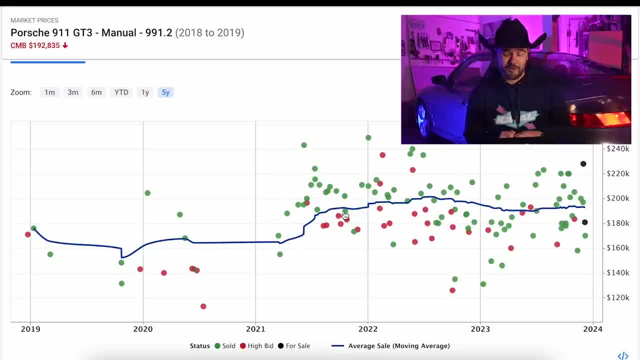 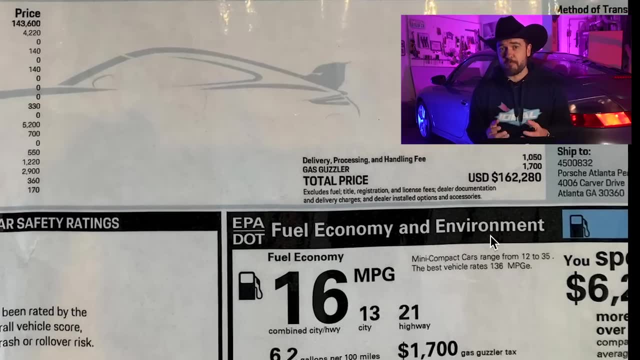 Plus and the market stayed hot for a little while. So let's take a look at this one. It's a blue GT3.. That is beautiful And, like that red GT3 bought pre-pandemic, this one was bought for. 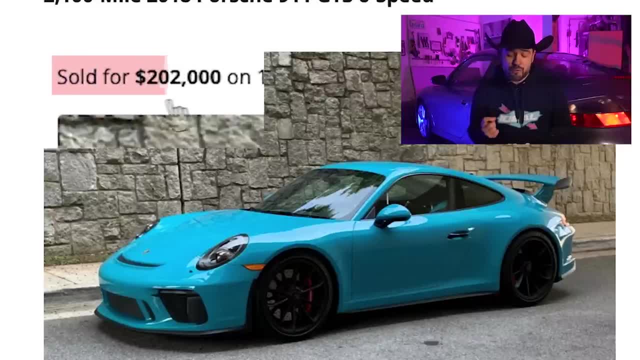 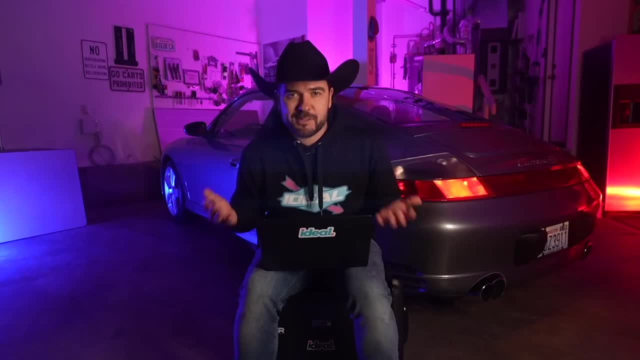 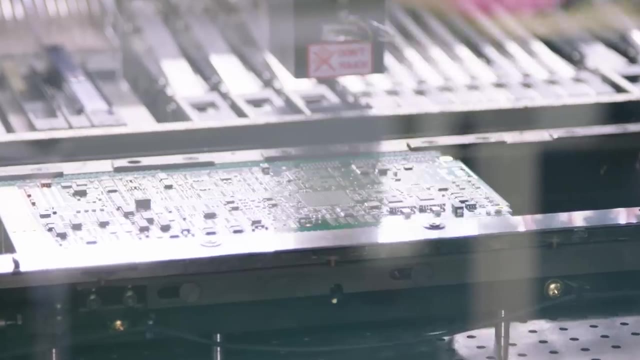 probably around $130,000 and sold for $202,000 plus fees. That's a $70,000 markup on a GT3. So it begs the question: well, how could this be happening? Well, remember the chip shortage being built. Well, the 992 GT3, the newest generation dealers were asking $100,000 ADM. 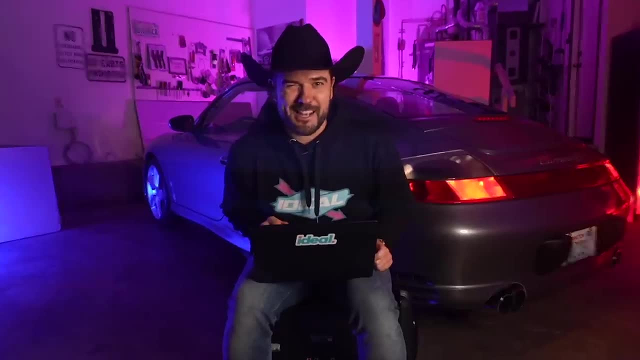 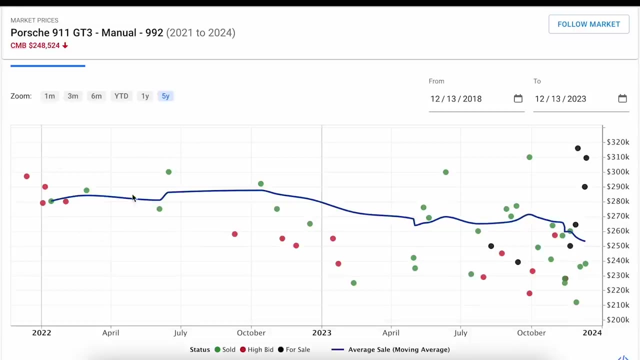 or additional dealer markup. So check this out. Here is your 992 GT3 chart And right off the bat you can see these cars started trading hands around $300,000 on average And MSRP on these started under $200,000.. So let's click into this one. That is a beautiful car with a $206,000 MSRP. 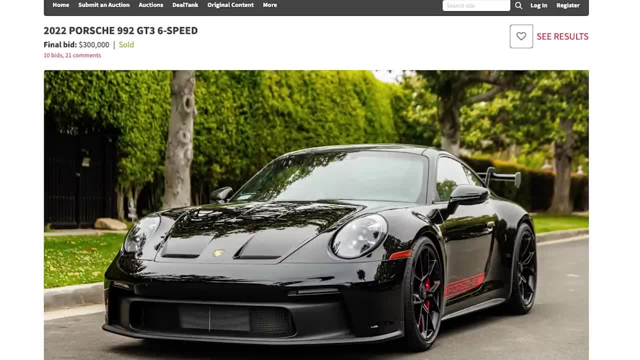 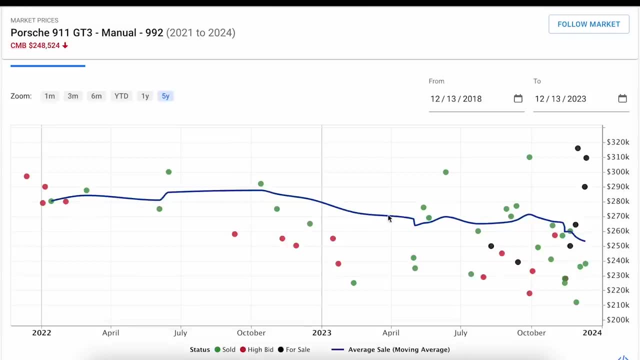 So when you factor in auction fees, this example sold for over $100,000 more than its original asking price. But as you can see, with this blue line the average sale price over time has been decreasing rapidly, with one just selling for roughly its manufacturer's suggested retail price. 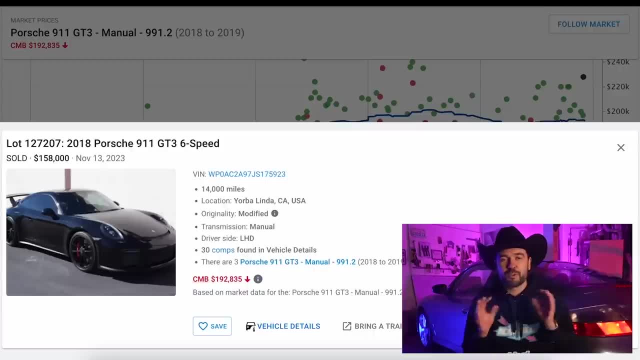 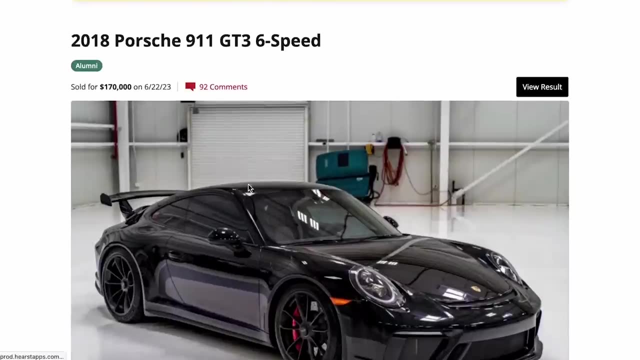 of $212,000, plus fees And guys, to really drive this whole thing home. let's take a look at this car that got sold not once, but twice this year. First, it was purchased on an auction site in June for $170,000. 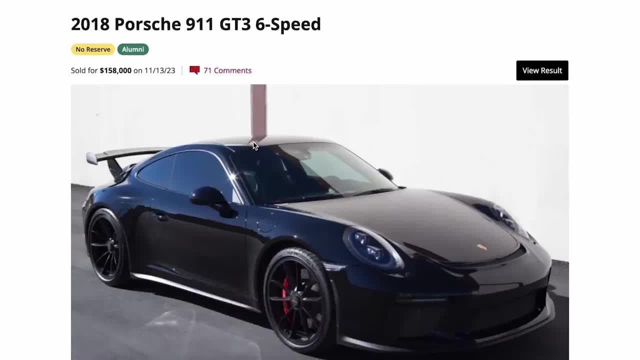 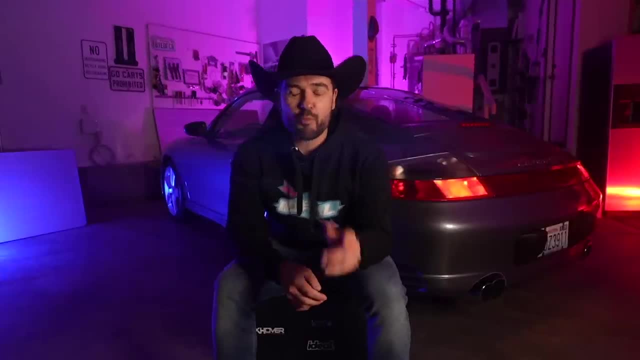 And it had 14,000 miles on it. Then, six months later, with the same exact mileage, it sold for $158,000.. So, guys, the market it's correcting, And cars, even special ones like the GT3s. 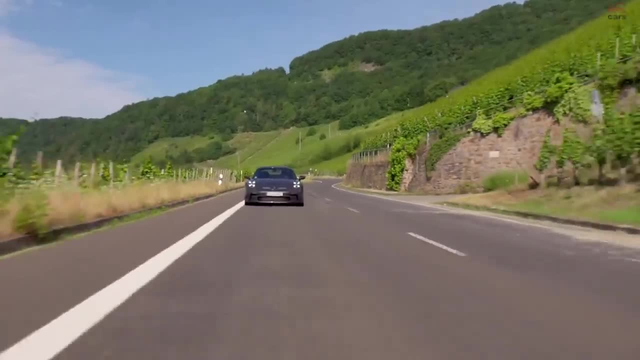 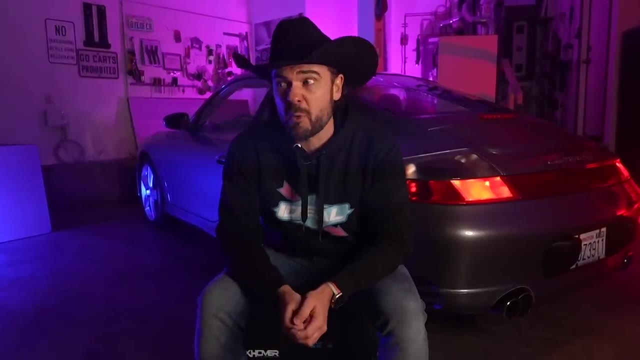 are depreciating like any used car should. So how come for a while there they didn't. Well, the pandemic really shortened the supply, So it made the GT3 become somewhat of a numbered car for a hot minute. See, when there is a limited supply, people well. 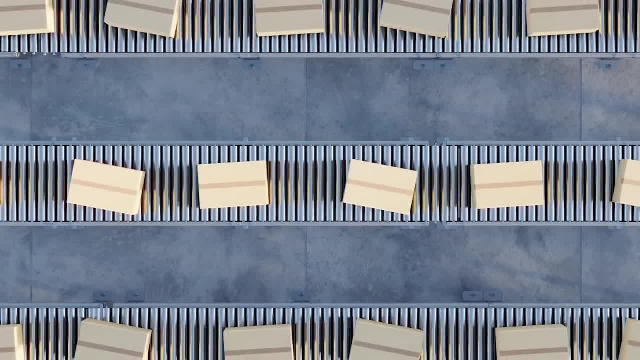 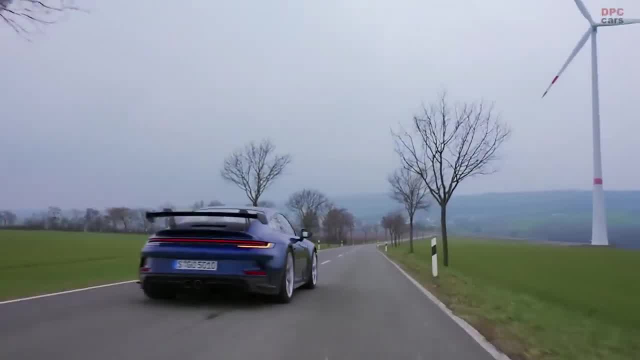 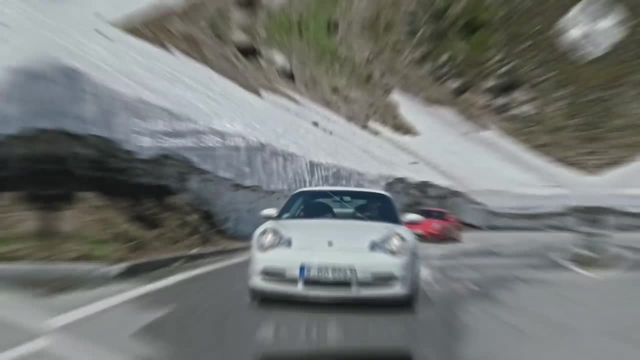 willing to pay more because they can get it today instead of getting it tomorrow or next year or the year after. But Porsche is laughing all the way to the bank because they're pumping out 3,000 plus GT3s and GT3 RSs per generation, which wasn't the norm with the 997 or 996 gen. So while they felt 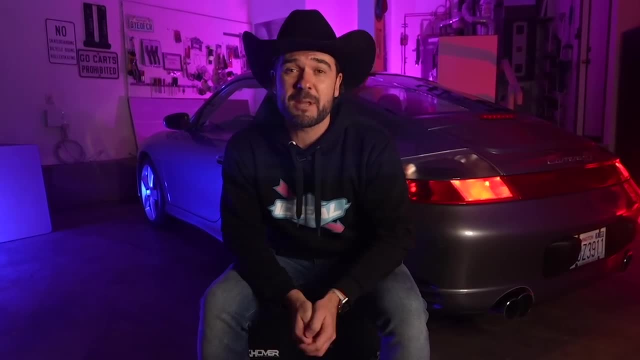 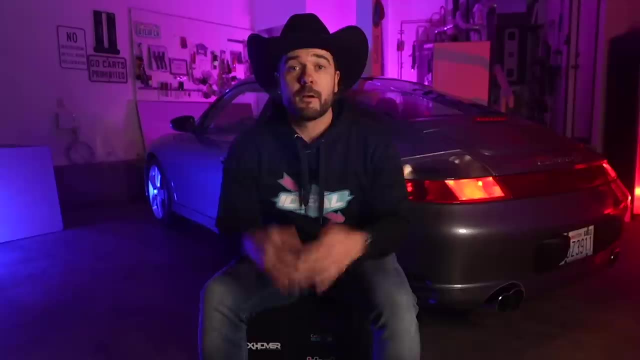 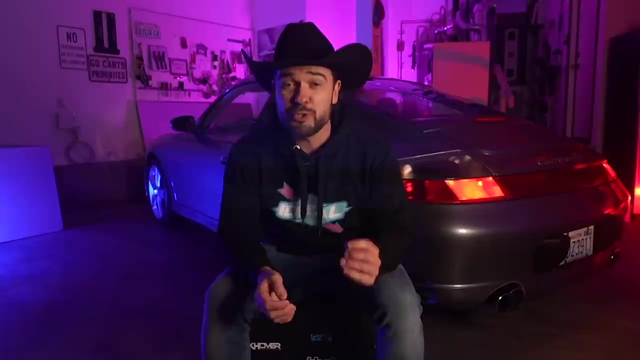 limited initially. once the chip shortage was figured out, the market became flooded with them for sale, Hence why you saw a huge spike in the number of cars transacting in 2021 on the chart, Also because of the markup of the 992 GT3 commanding a $100,000 premium, the older 991.2 GT3, which is essentially 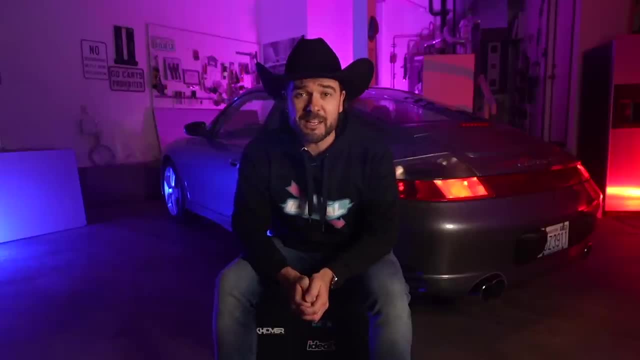 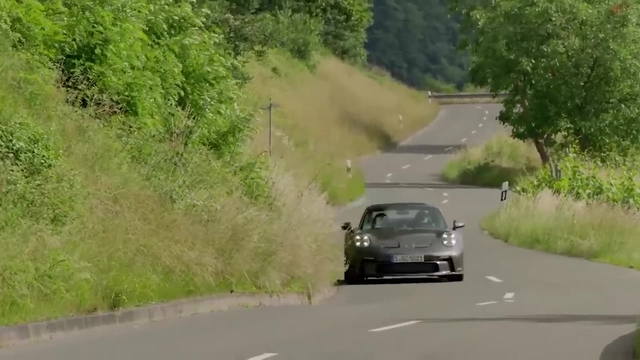 the same car went from a car sold for under MSRP to a car that was 10 to 15% cheaper and more available to purchase than the 992.. Now that $100,000 markup on GT3s had a trickle-down effect, 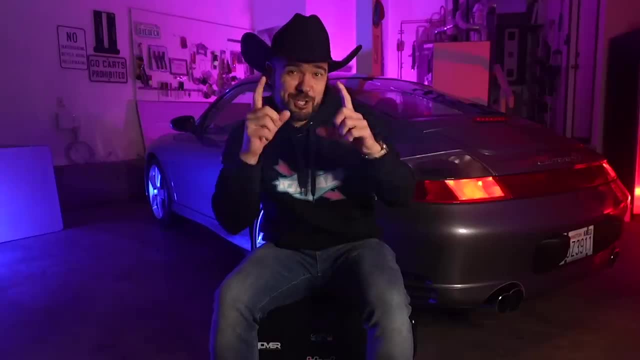 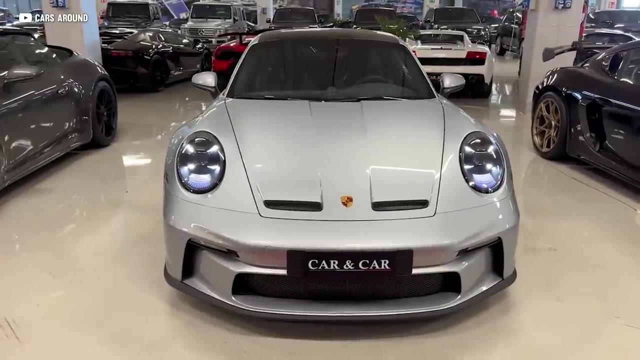 that all 911 buyers had to endure. Okay, so picture this: You're sitting down in a showroom and this beautiful $200,000 GT3 is staring at you, But the dealer, they want $300,000 for it. So now, when a shopper's going in there to buy a 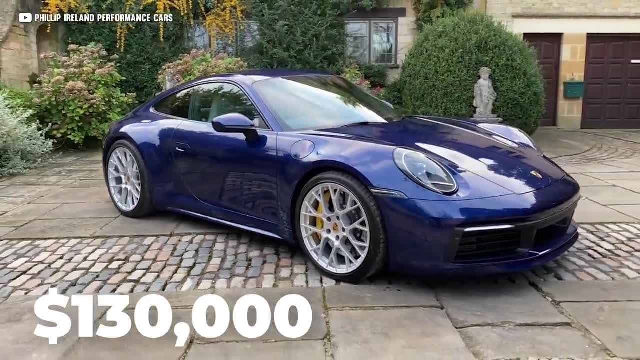 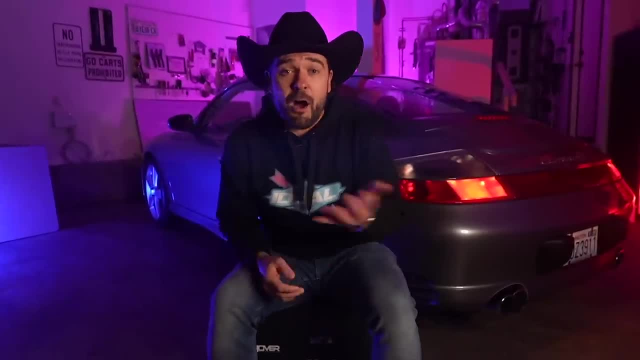 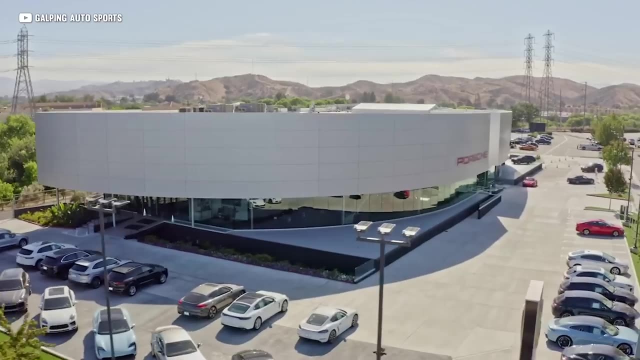 Carrera S for $130,000, when there's only an asking of a $10,000 markup for the right to buy that car sounds like a steal of a deal. It made the lesser models sell like hotcakes because, with very limited supply, paying a slight markup to have it today felt like a no-brainer And even 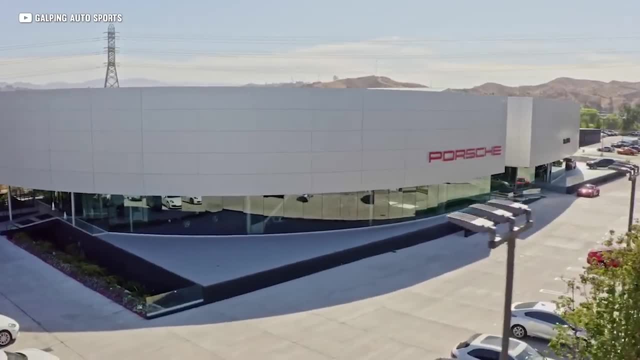 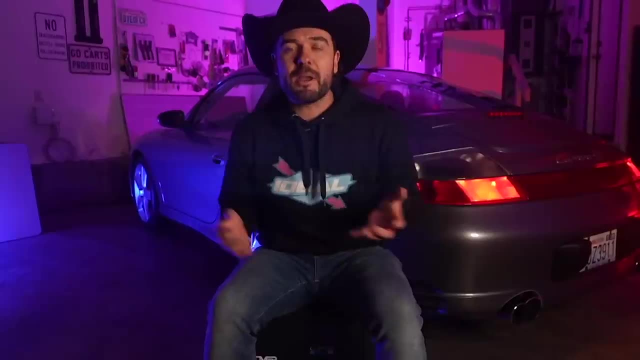 dealers used this to their advantage, hiking prices even on cars that weren't hot sellers, which played with our minds and gave us a lot of money. That's a higher perceived value of a car's desirability. Also, it added pressure to buyers. 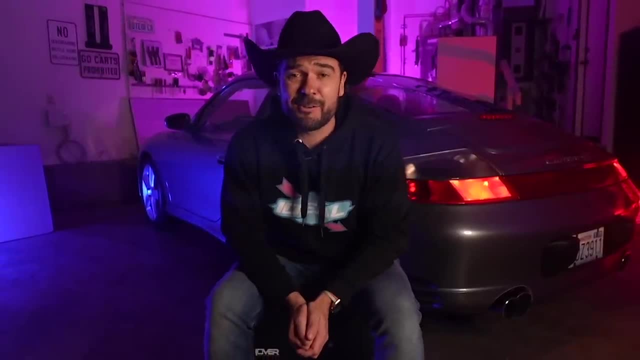 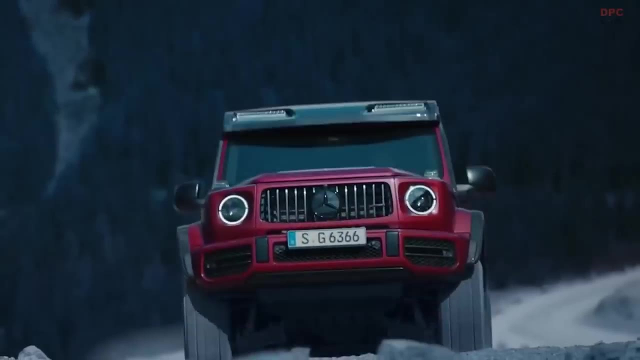 to make us feel like if we decided to pass on a specific car, well, there was no chance that we would be able to find another one anytime soon. And, like I said, it wasn't just Porsche. We saw this with Mercedes when they were asking $100,000 over MSRP to buy a new G-Wagon, And then their 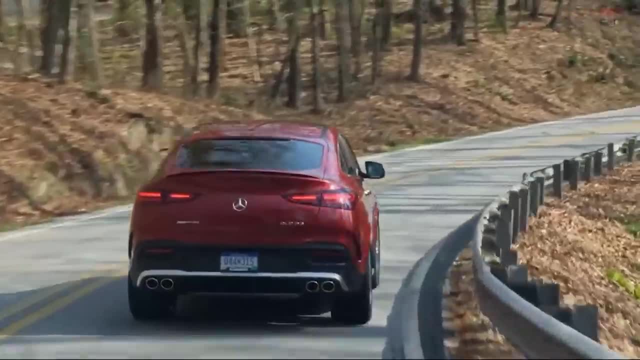 mid-tier GLE, well, with a slight markup, sold, sold, sold. Or even Ford with the Bronco Raptor with a $72,000 MSRP that we're selling for $130,000.. So that's a lot of money. 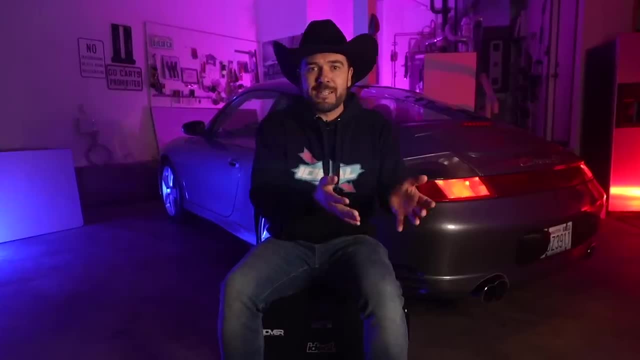 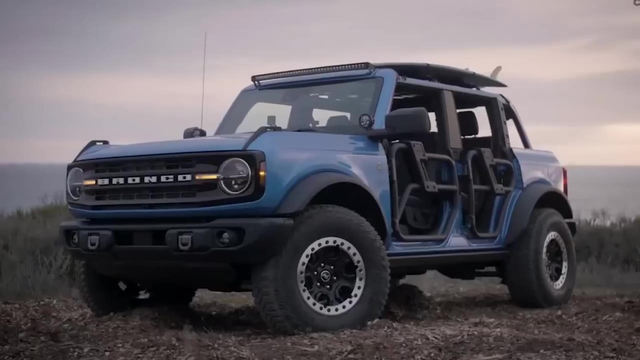 So you'd go into the Ford dealer. you see that thing for $60,000 over. and now all of a sudden that Bronco Sasquatch with a $10,000 over markup. again, buyers felt like they were getting a deal. 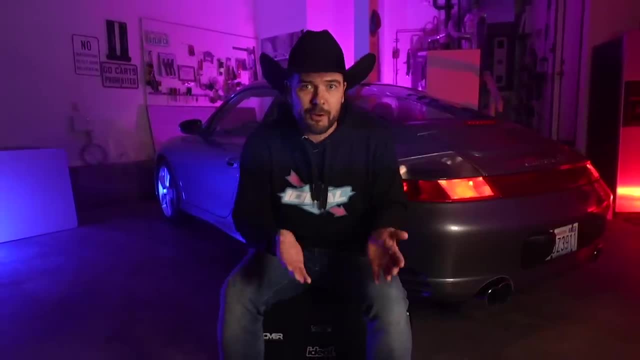 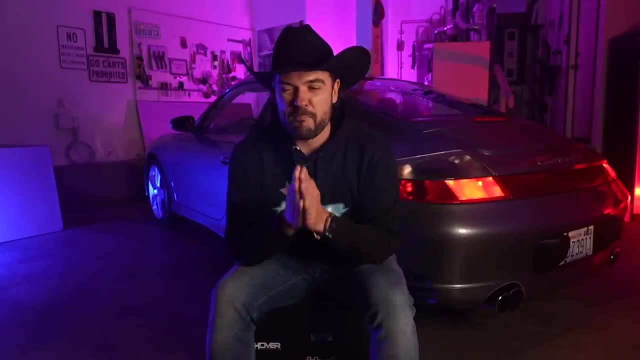 Everyone was selling cars for markups, which is why we hit a record high of almost $50,000 for average new car prices. So today, yes, there were four big things that happened to get us to where we are today. First was the impact of economic factors. You see, 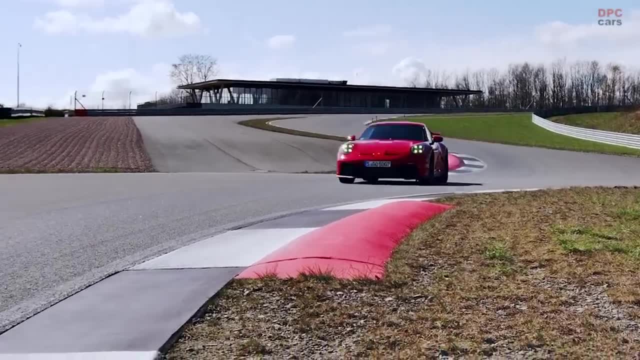 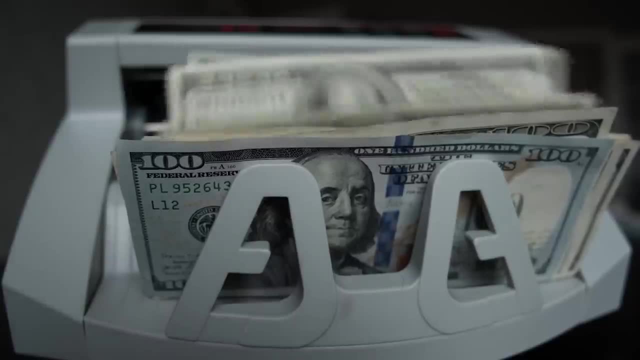 demographic interested in Porsche. particularly high-end models like the GT3s, the GT3 RSs and the GT4 RSs are the most affected by the rising interest rates and tech industry layoffs. These economic pressures directly affect the demand for luxury cars. Second is Porsche's 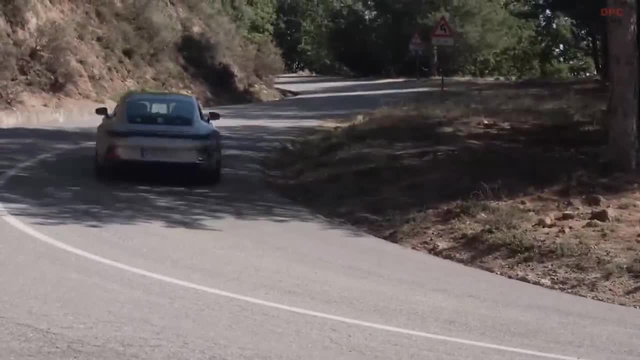 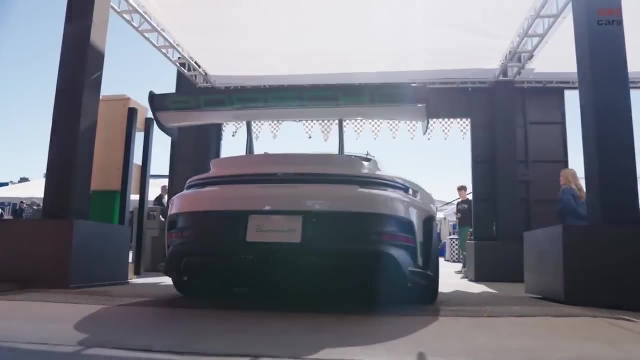 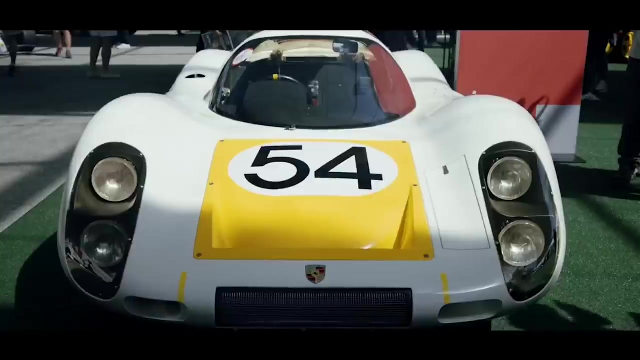 production strategy, Porsche has been releasing more cars in different versions, like the Spyder and the RS models. This approach seems to aim at curbing speculation and encouraging purchases based on enjoyment rather than investment potential. Third is Porsche's brand philosophy. I mean Porsche, they're going back to their roots and 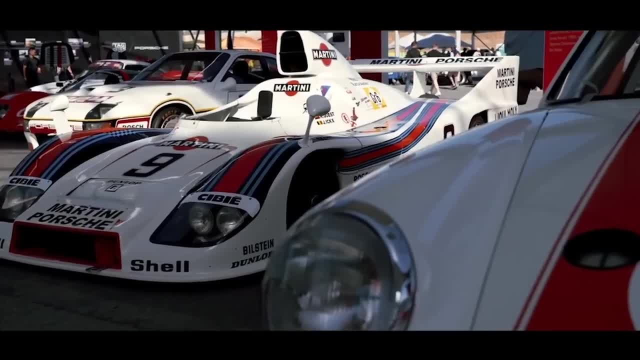 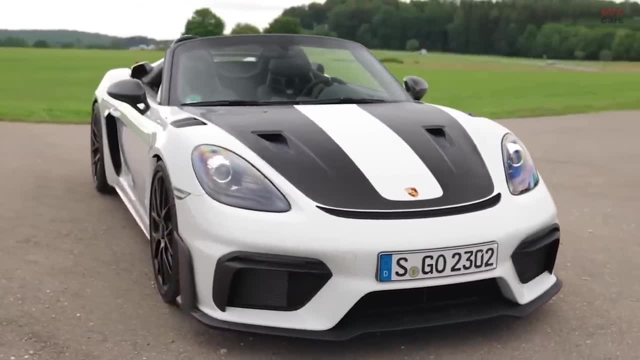 what made them absolutely great. They want to be known for making cars for enthusiasts and actual users, not just investors or speculators. I mean, in recent years there's been a trend of people buying Porsches only to resell them for higher prices, often without even using them, I mean. 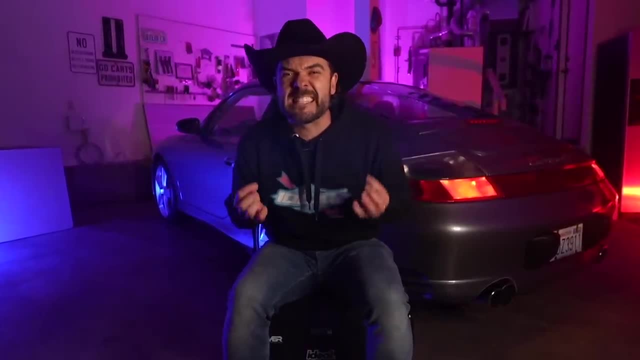 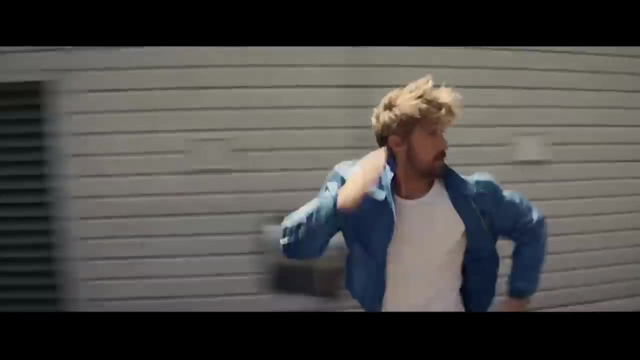 look, there's cars out there that they haven't even taken the plastic off the seats yet. And lastly, it's great for us enthusiasts today because it's a shift towards true enthusiasts. Porsche's strategy of releasing various versions of their models appears to be an 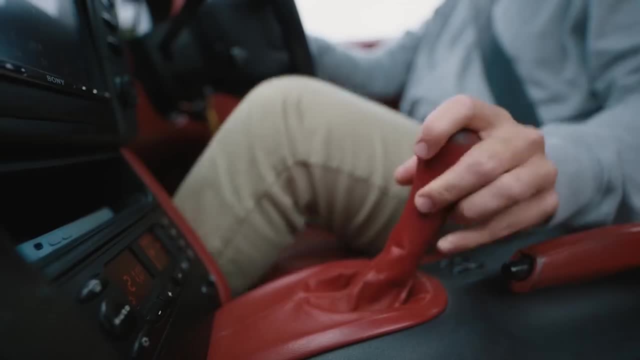 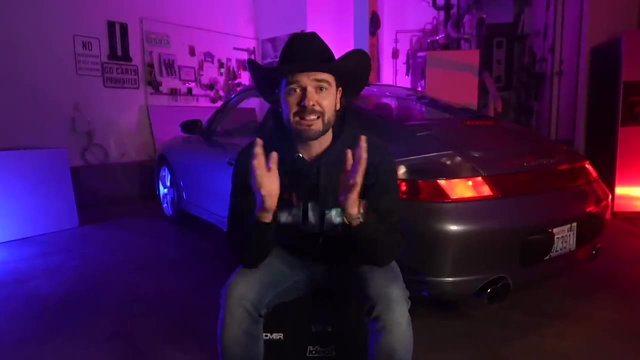 effort to attract real car enthusiasts back to their brand, moving away from the buyers, who treat their cars purely as investment opportunities. So, guys, to sum this all up, Porsche, a leader in the enthusiast market, is shifting away from building investment quality, limited edition cars. 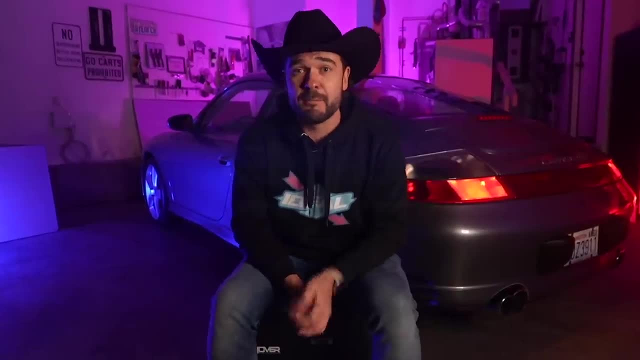 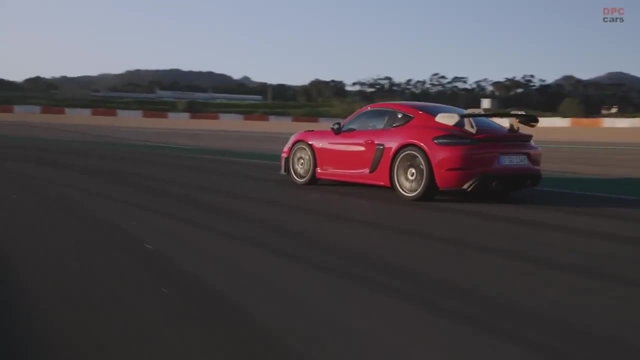 to a more unlimited production of each variant, meaning they will depreciate. Yes, it's awesome. for any enthusiast like you and me, It's the start of a market. It's the start of a market. It's a monumental shift to pre-pandemic pricing. It's going to encourage owners to get out there. 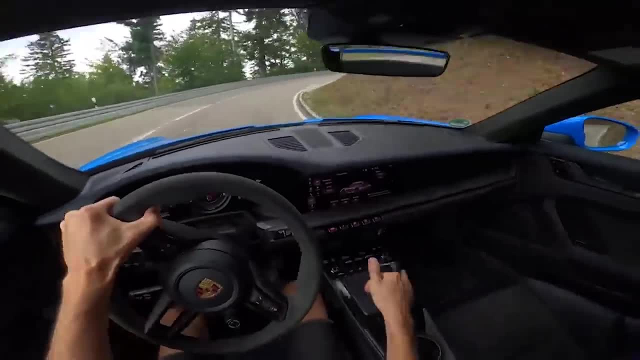 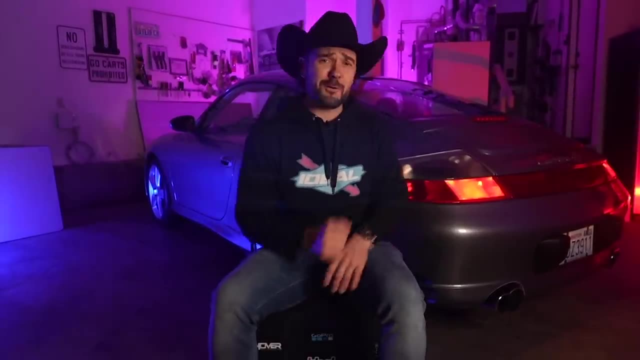 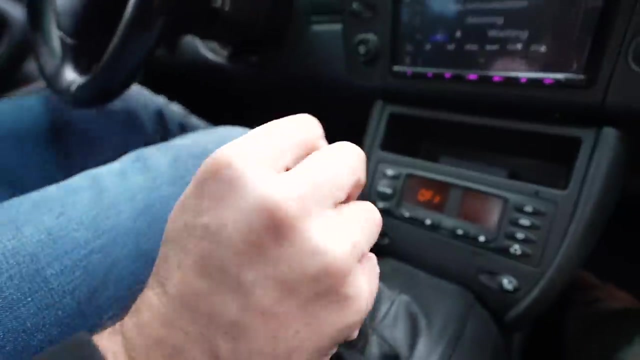 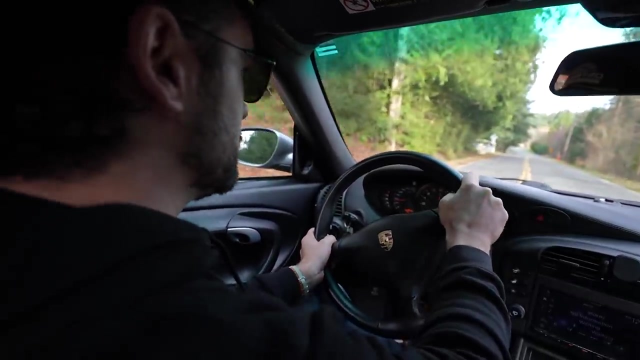 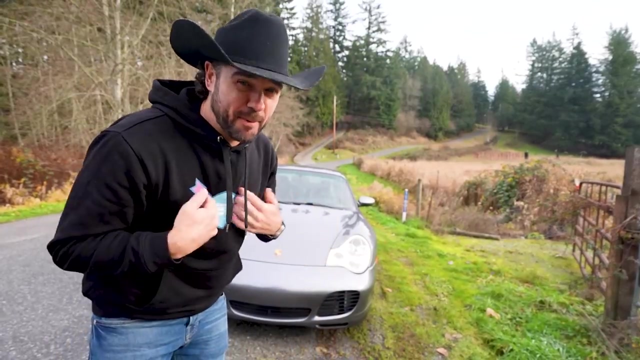 and drive them, instead of treating them like a garage queen investment, which is exactly what they were built to do- Well, not the garage queen part. So why don't we go for a quick drive Now, guys? this is the 996 C4S that I bought pre-pandemic for 19,500 bucks, And now they're. 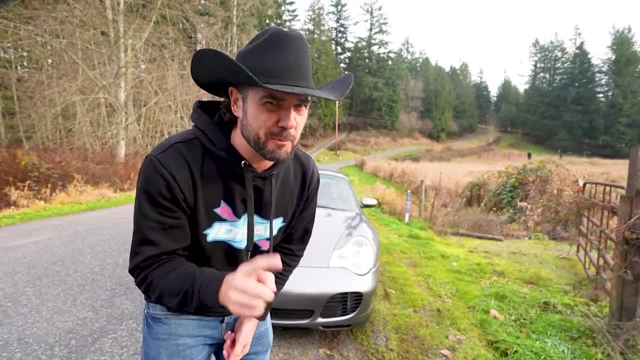 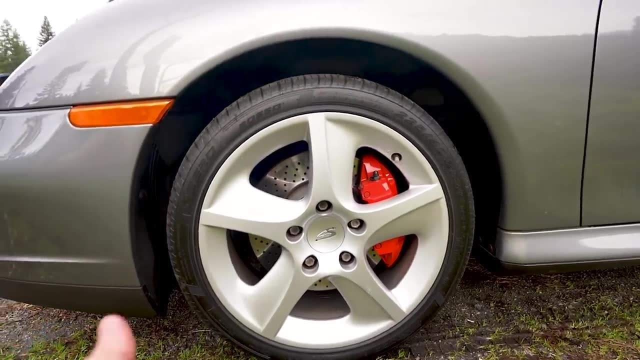 trading hands for double that. But real quick, let me show you around what a $40,000 Porsche looks like. First up, since it's a C4S, you got the brakes from a turbo and these awesome five-spoke alloys. Inside you even got Bose sound. You got some well pretty good looking leather. 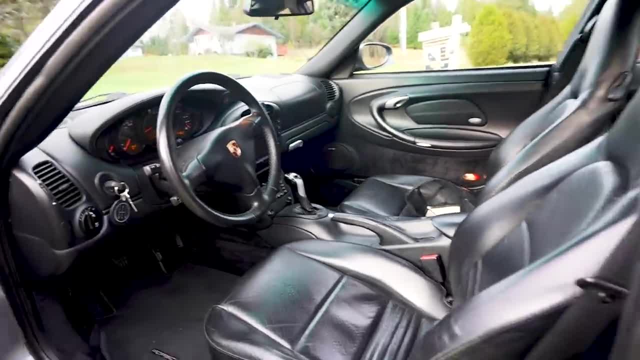 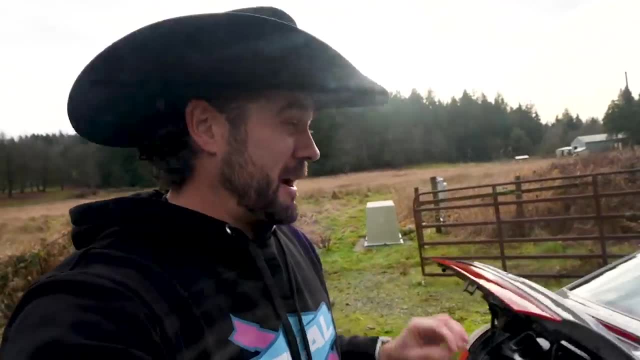 85,000 miles on the odometer, And I'm going to show you what's in the box: A pretty dated interior. Now for the business end. oh, four liters of fury. Yes, The crazy thing about this specific car is it actually has a four liter. because, well, these cars have bore score and IMS RMS issues. So LOL, right Now is this a $40,000 car? I don't know. I mean realistically it doesn't drive like a $40,000 Porsche, but that's what they're trading. 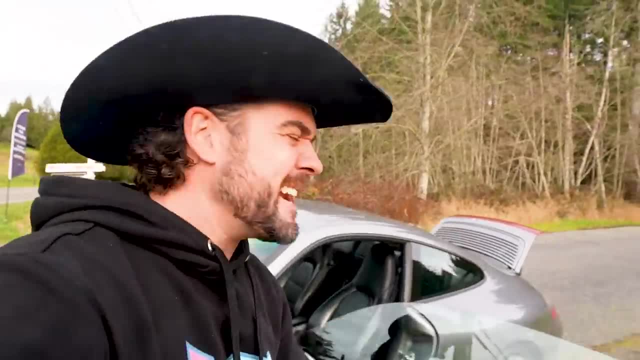 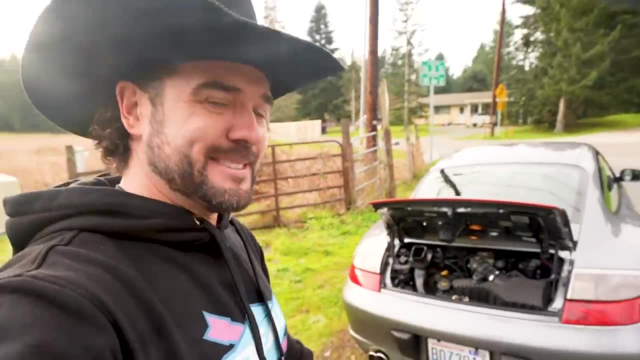 hands for now. So if the top of the market, you know the 992s, the 991s and even the 997s, start to come down in price once again, the starter Porsche like this one, yeah, it's going to be more than attainable. And guys, 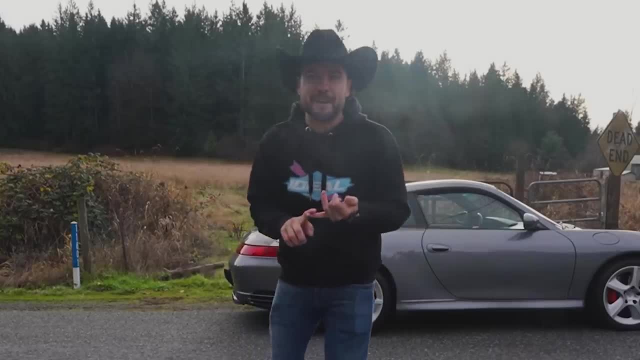 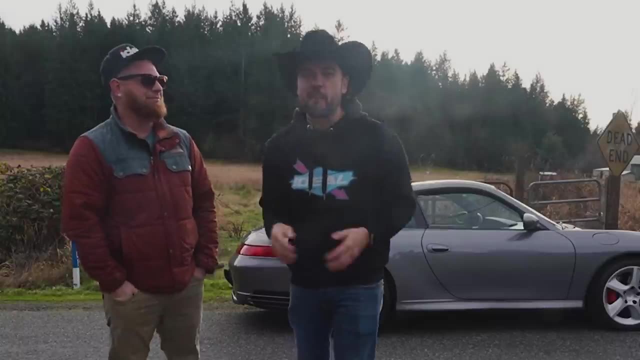 that's what being a car enthusiast is all about. It's about driving, enjoying and connecting with fellow enthusiasts like this guy right here. It's not about bragging about how much money you're going to make on your ride by not driving it. It's an exciting time to love cars.